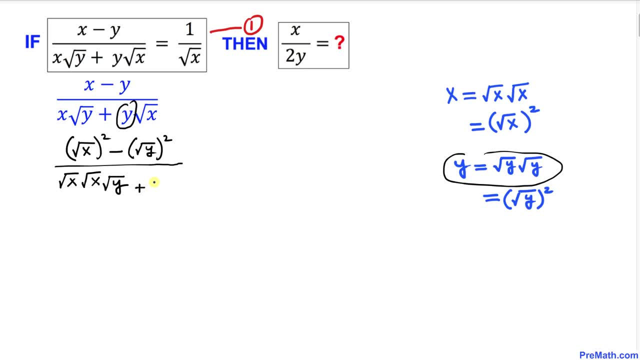 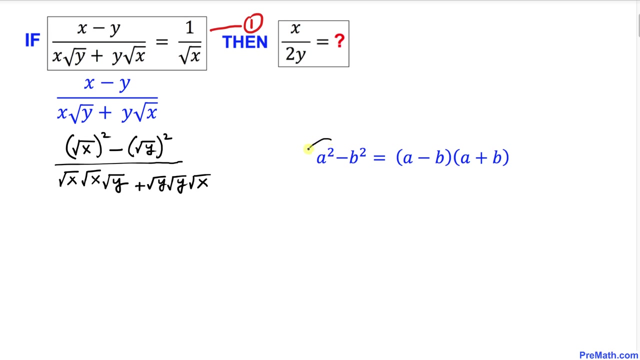 written as square root of Y times. square root of Y. I can write this one as square root of Y times. square root of Y times. this square root of X. now let's focus on the numerator we can see over here. this represents the difference of two squares. therefore, we are going to use this formula: a square minus B square. so 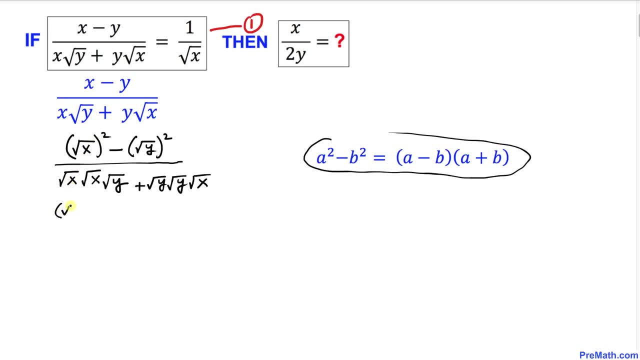 this could be written as simply: square root of X minus the square root of Y, times square root of X plus square root of Y. now let's focus on the denominator. we can see that the square root of X is in common between these two terms, and square root of Y is in common as well. therefore, I can factor. 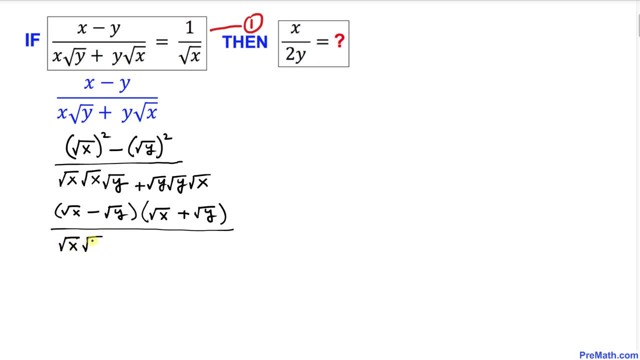 out square root of X times square root of Y. outside and parentheses, we ended off with square root of X plus square root of Y, and now we can see that this and these factors they cross out. so we are ended up with square root of X minus square root of Y, divided by square root of X times square root of Y. and since we 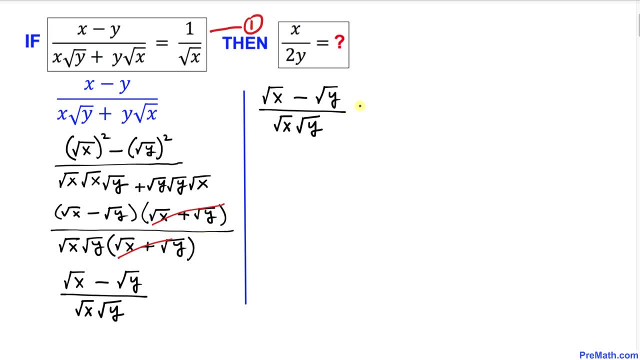 are running out of space on the left hand side. I have just moved on this right hand side and now we can write this fraction as square root of x divided by square root of x times square root of y, minus square root of y divided by square root of x times square root of y, by using: 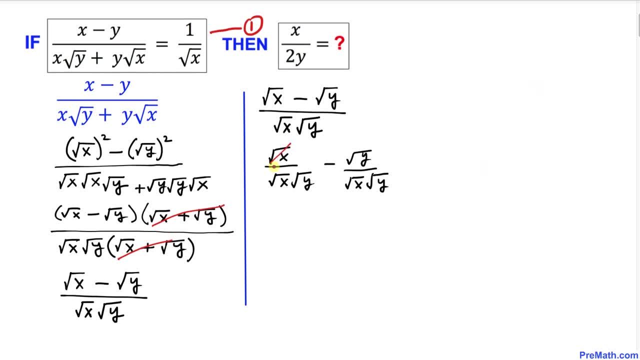 this fact, and here we can see we can cross out these ones and here these ones and here one as well. so i can write this one as a 1 over square root of y minus 1 over square root of x. so our equation number one is going to become simply: the left hand side has been simplified. 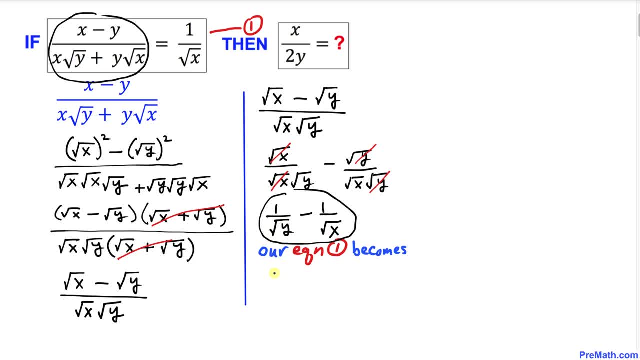 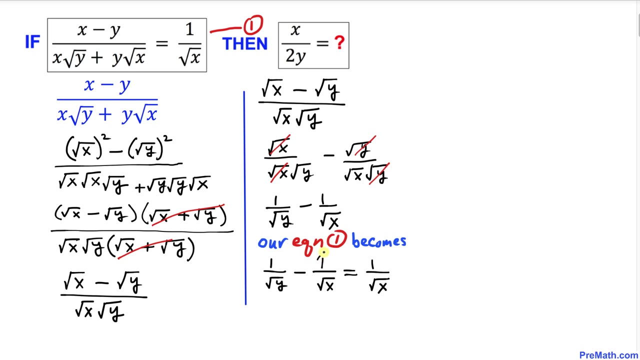 to this one. i can replace the left hand side as 1 over square root of y, minus 1 over square root of x. equals to the right hand side, is 1 over square root of x. and now let's go ahead and move this negative 1 over square root of x on the right hand side, and here, 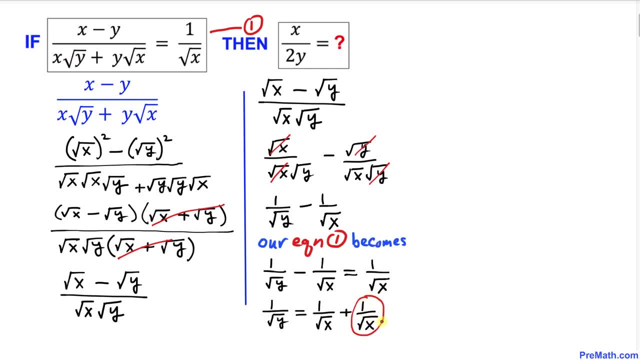 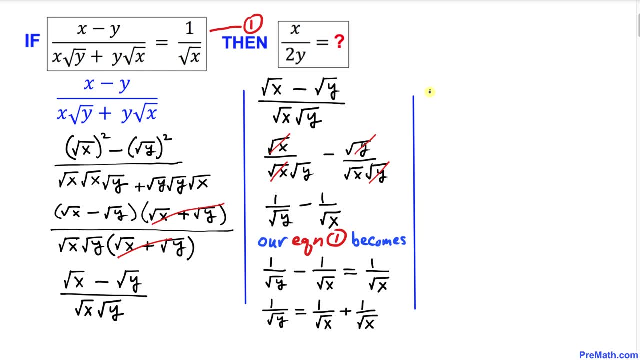 1 over square root of x has been moved to the right hand side. and now let's go ahead and combine these two fractions on the right hand side, so our equation is going to become: 1 over square root of y equals to 2 over square root of x after adding these two fractions. and now let's go ahead and. 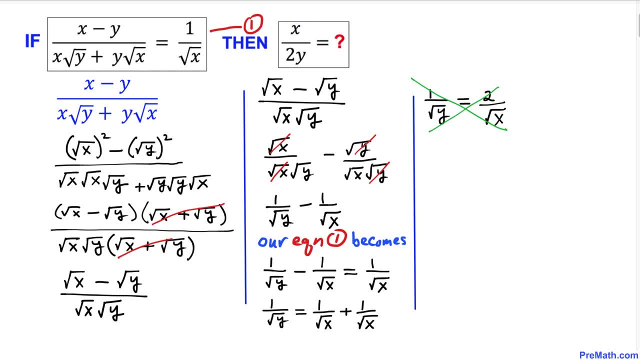 cross multiply to remove these fractions. and now let's go ahead and cross multiply to remove these fractions. and now let's fractions. so that is going to give us 1 times square root of x, is going to give us square root of x equal to 2 times square root of y. now let's go ahead and remove these radicals by taking the. 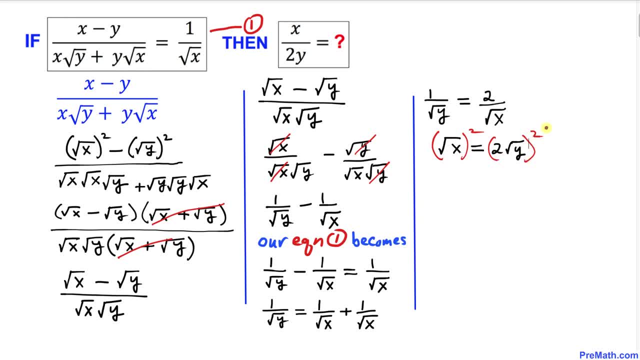 squares on both sides. so on the left hand side, this square and square root- they undo each other. we got x equal to this. 2 square is going to become 4 times this square and square root- they undo each other- becomes y. so thus we got x equal to 4y. and here's our final step. let's go ahead and. 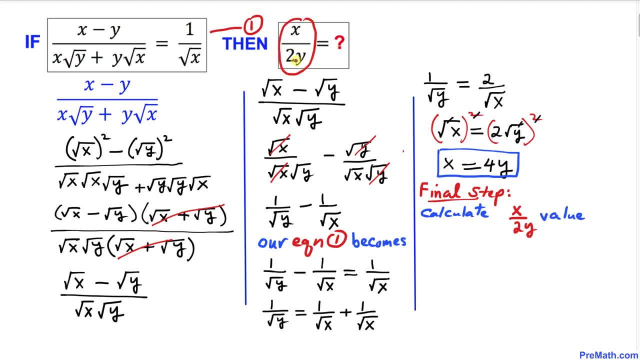 calculate the value of x divided by 2y. and here i have copied down x over 2y. let's go ahead and fill in the blanks. x, in our case, is 4y, so the numerator x could be replaced by 4y divided by. we are just going to write down 2y. 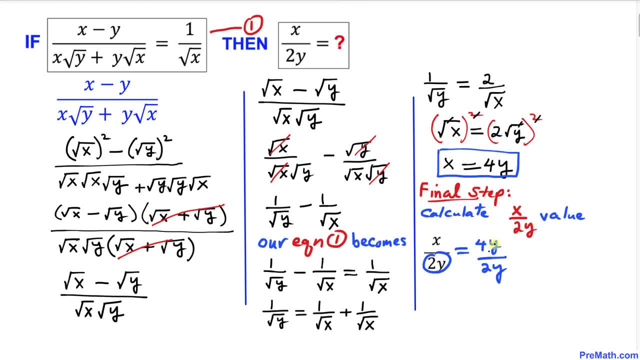 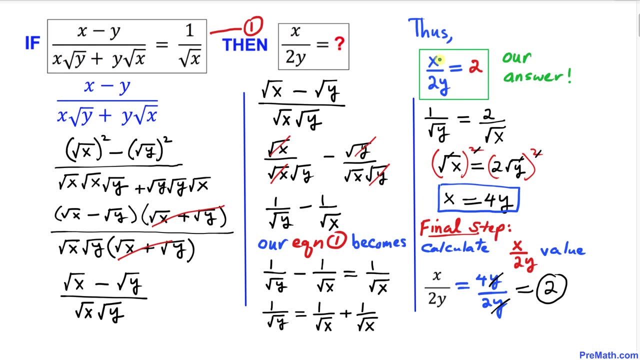 and we can see that this y and y cancels out, and 4 divided by 2 is going to give us 2, so that means x over 2y turns out to be equal to 2, so thus our x over 2y value turns out to be 2. 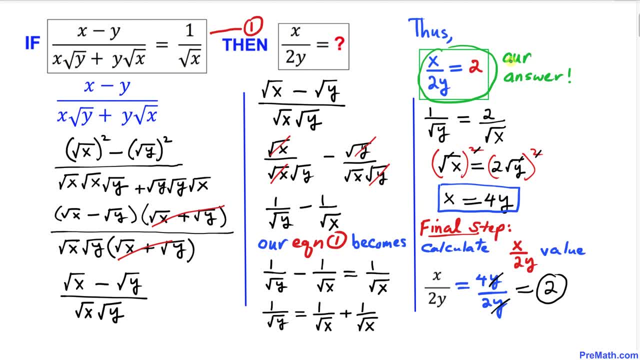 thanks for watching and please don't forget to subscribe to my channel for more exciting videos. bye.